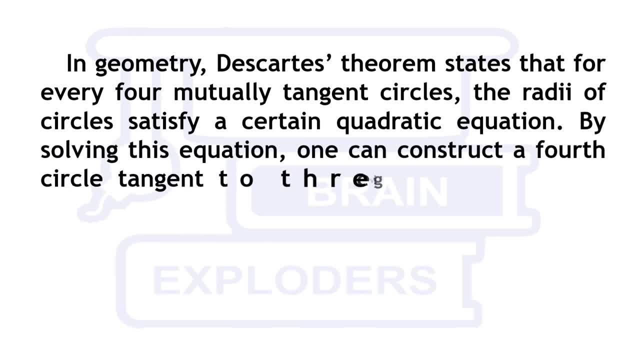 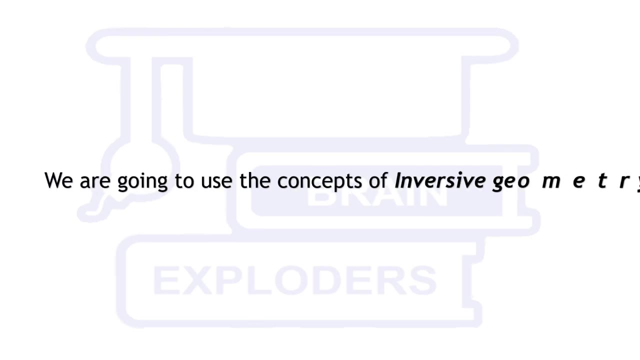 radii of circles satisfy a certain quadratic equation. By solving this equation, one can construct a fourth circle tangent to three given mutually tangent circles. Theorem is named after René Descartes, who stated it in 1643.. In this video we are going to use some basic concepts of Inversive Geometry. We have already 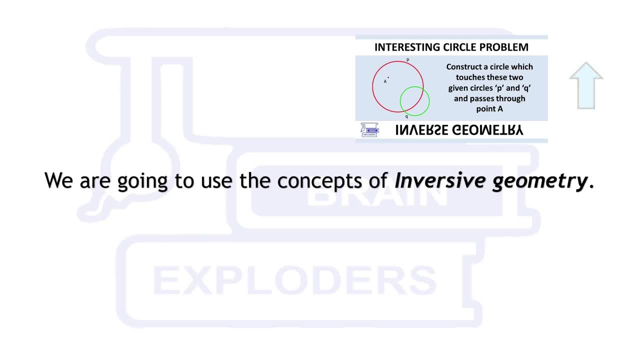 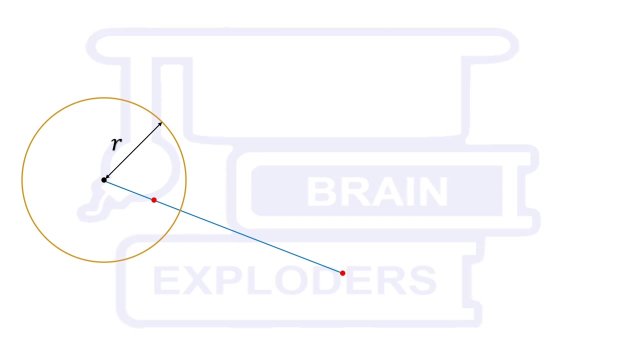 made a video on Inversive Geometry. The link of the video is given in the i button. The circle about which we do the inversion of any point in the same plane is called reference circle. All the points inside reference circle have their inverse outside the reference circle, and vice versa. Let the radius of reference circle is r and. 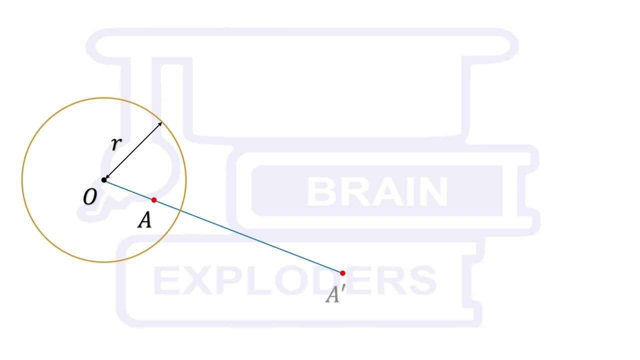 there are two red points, one outside and other inside the circle, which are collinear with the center of reference circle. These two red points are inverse of each other. if, and only if, product of their reference circle. If, and only if, product of their reference. 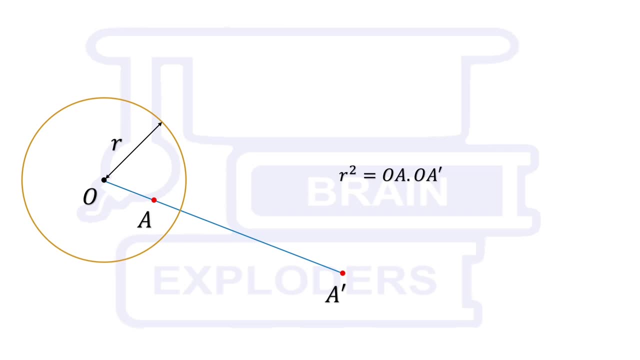 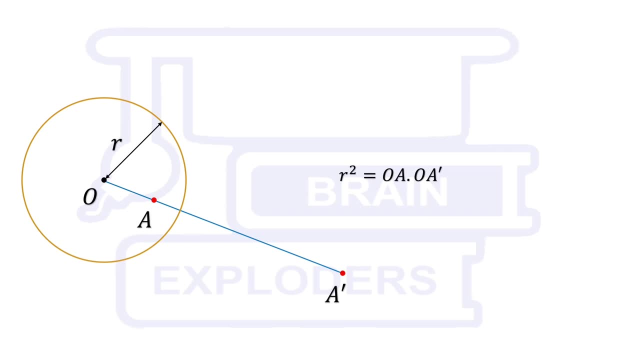 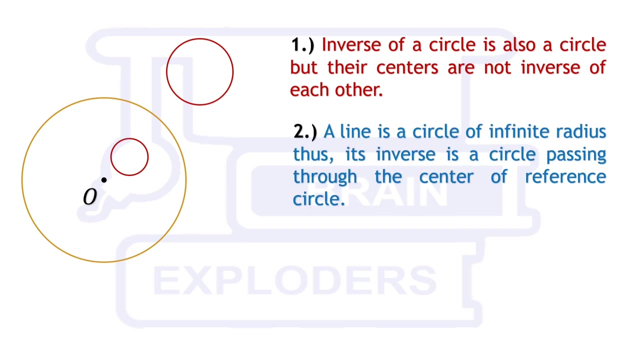 is R squared. If we find the inverse of all the points of a curve, we obtained another curve which is called the inverse of the previous curve. Inverse of most of the curves have different shapes, but inverse of a circle is another circle, Since line can also be considered as a circle of infinite radius. therefore its inverse. 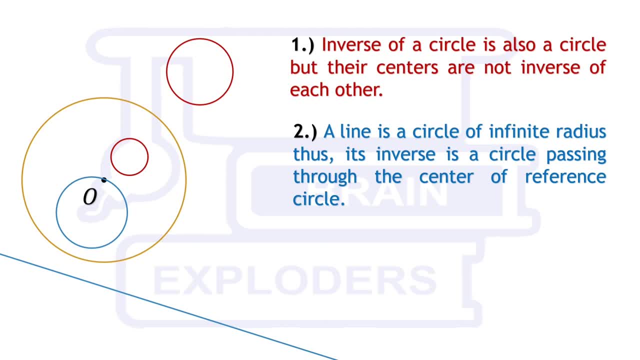 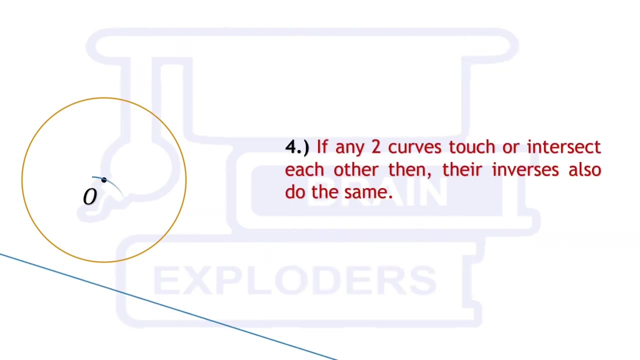 is also a circle which passes through the center of reference circle. If any curve touches or intersects reference circle, its inverse also touches or intersects the reference circle. Moreover, if any two curves touch or intersect each other, then their inverses also do the 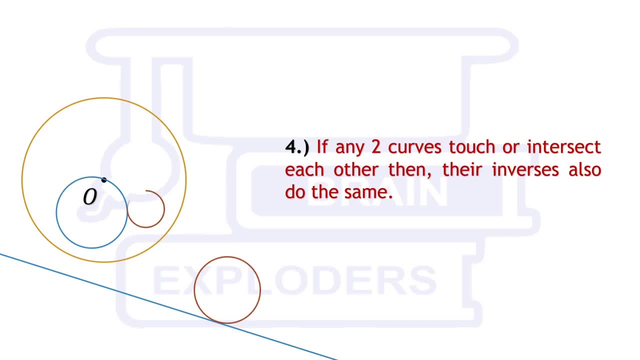 same with each other. You can see that brown circle touches the light blue line and its inverse is also touching the inverse of this blue line. Similarly, if we assume red and blue lines are the circle of infinite radius, they intersect each other twice: one time as shown on the screen and other time at infinity. 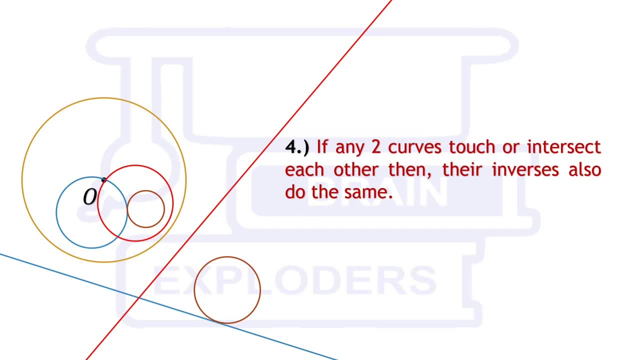 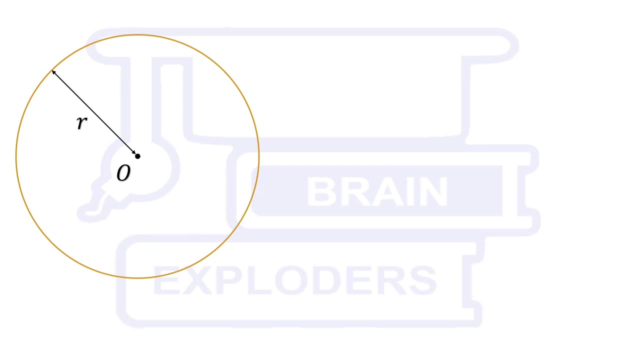 Therefore their inverses are also intersecting each other two times, in which one of the two circles are intersecting each other twice. Let's see what is the relation between the radii of the circles which are inverse of each other. Suppose center of one of the circle is at a distance of a from o and its radius is r1.. 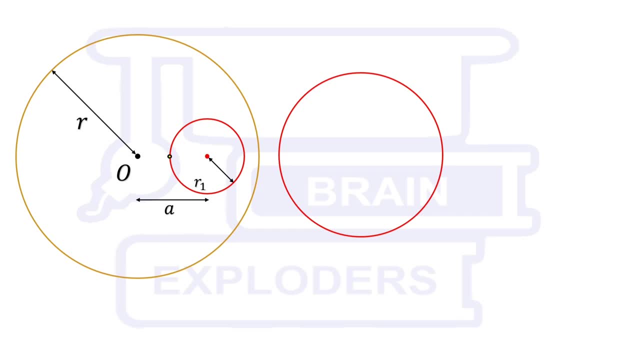 If a is the point on this circle which is nearest to o, then a' must be the point on inverse circle which is farthest from o. So r2 must be equal to oa times oa'. oa is equal to a-r1, we get oa' equals to r2 over. 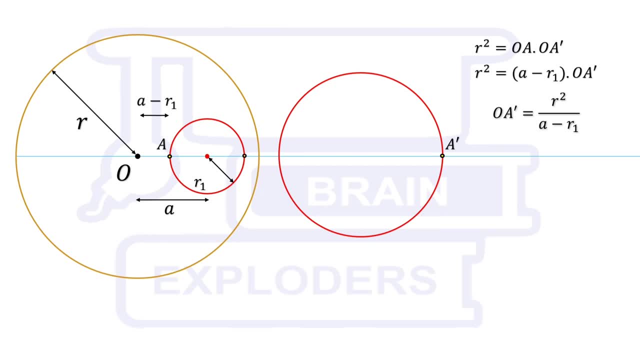 a-r1.. Similarly, inverse of b is b' and ob' is equal to r2 over a plus r1.. a'b' is the diameter of the inverse circle. Therefore, twice of capital, R1 is equal to r2 over a plus r1.. Similarly, inverse of b is b' and ob' is equal to r2 over a plus r1.. a'b' is the diameter of the inverse circle. Therefore, twice of capital, R1 is equal to r2 over a minus r1.. 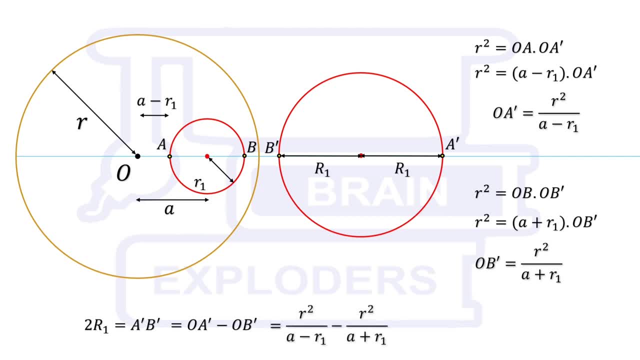 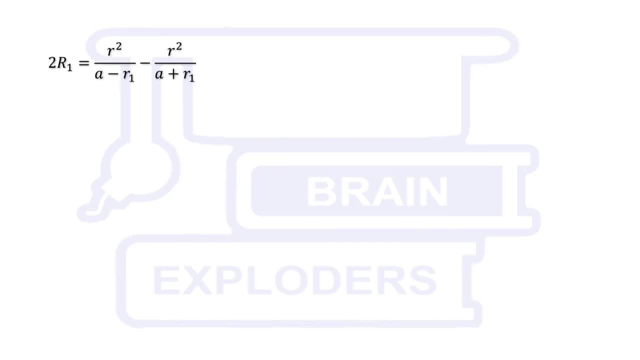 On substituting the values of oa' and ob', we get 2 times r1, equals to r2 over a minus r1, minus r2 over a plus r1.. Later we will need the value of reciprocal of this radius. therefore it is further solved. 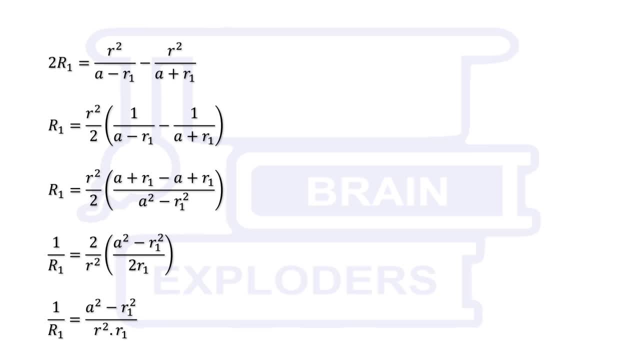 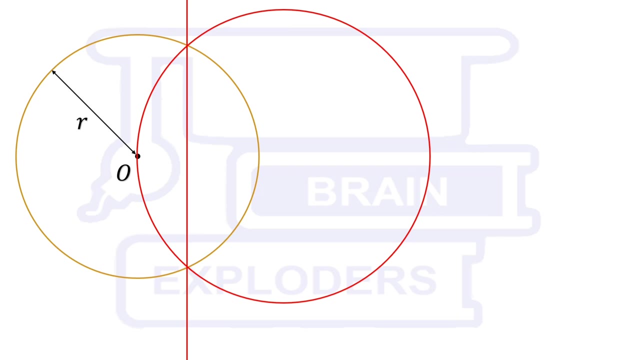 upto 1 over r1.. Now we are going to find the radius of that circle which is inverse of this line. The line intersects reference circle, so its inverse also intersects the reference circle. at same points, Since it is a line, its inverse pass through the center of the reference circle. 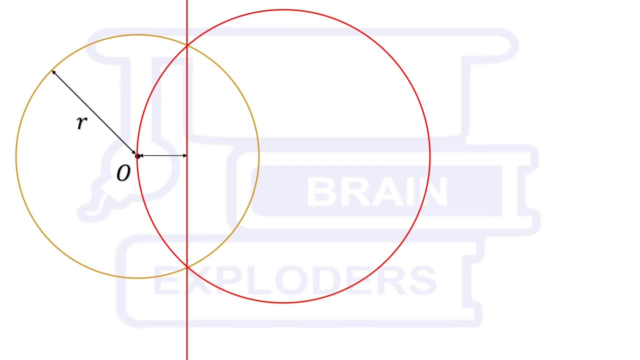 These three points are sufficient to predict the inverse of this line. Again, if A is the point on this line which is nearest to O, then A' is the point on inverse circle farthest from O, and A' must be the inverse of A. 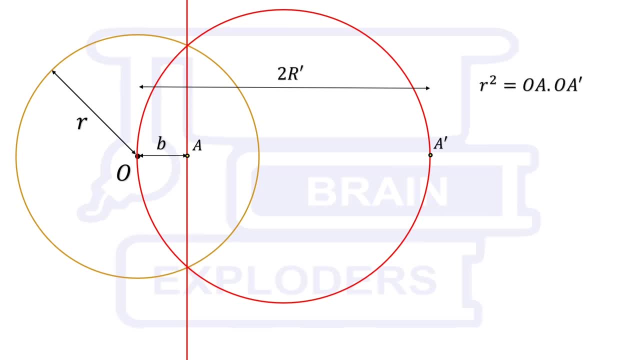 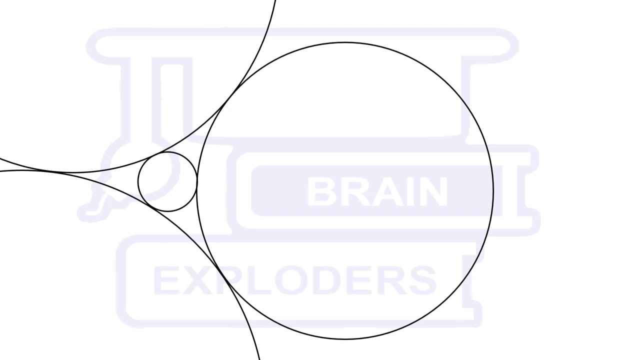 Here also, R squared is equal to OA times OA'. On substituting the values of OA and OA' we get 1 over R' equals to 2B over R squared. Here comes the most important section of this derivation Suppose. these are the four mutually tangent circles, relation between whose radii is to: 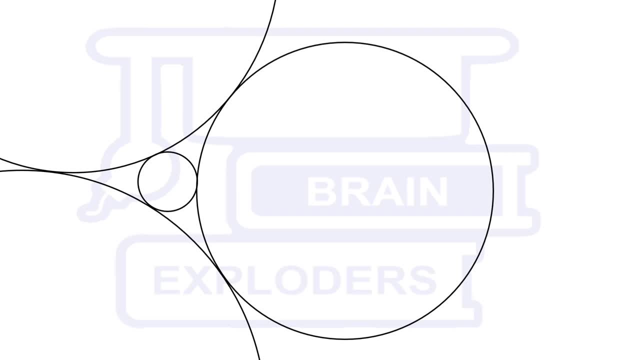 be find. Let us assume a reference circle for the inversion of this system, whose center is O. We have to take this circle somewhere such that O lies on any of the touch point. Make the inverse of all these circles, one by one. Since two of the circles pass through center, their inverses are lines parallel to each. 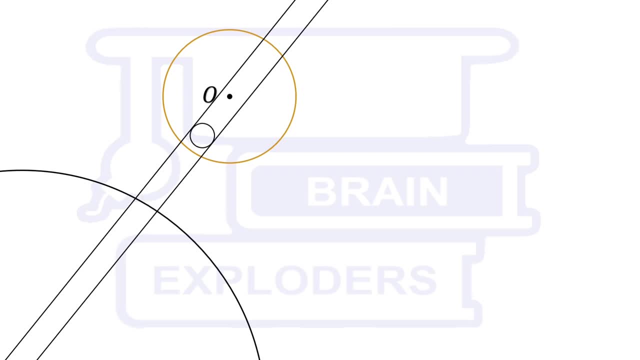 other Inverse of other two circles are circles, but both of them must touch each other, as well as both the lines. When we take the inverse of these four elements, we again find the previous system of four mutually tangent circles, No matter what is the distance between parallel lines. the inverse of these four elements. 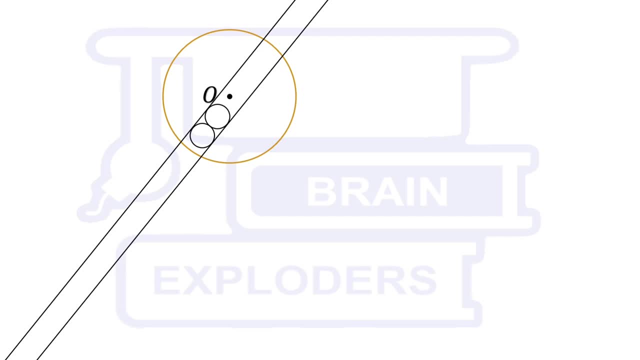 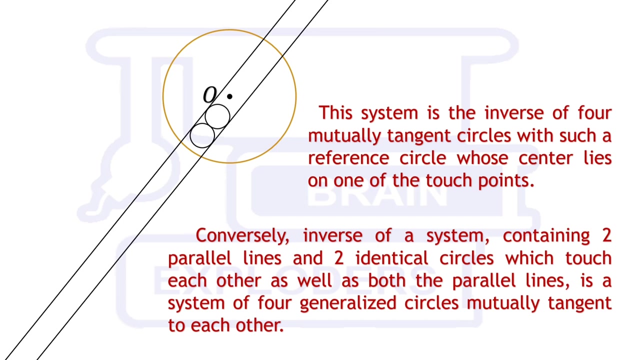 and the distance between parallel lines. and where the two identical circles are taken, inverse of this system will always be four mutually tangent circles. So let's generalize this system with some parameters, find the radii of inverse of these elements in terms of those parameters and eliminate the parameters to find the relation. 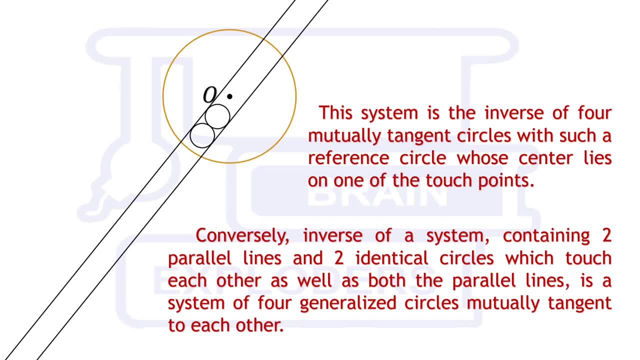 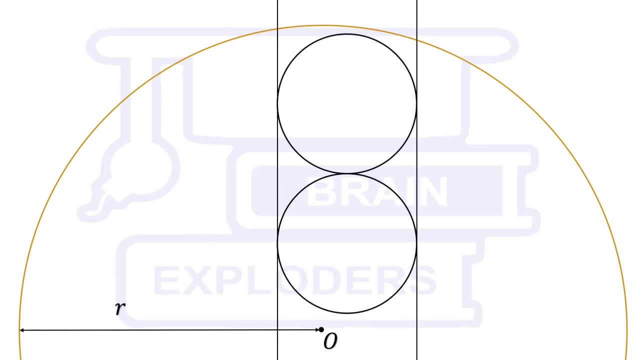 between their radii. Suppose this is the reference circle of radius R and center O. Here are two circles. Here are two circles and two parallel lines for our help. Parallel lines are considered strictly vertical and are at distance of A and B from O. 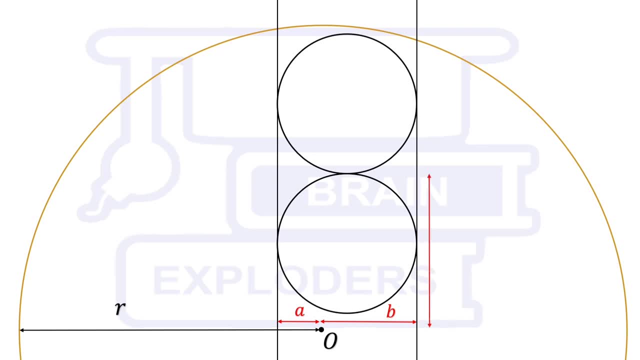 Point of contact of the two circles is C by 2 units above the center of reference circle. Obviously, this point and O are not lying on same vertical line. You can also take C in place of C by 2.. But later you will find that C by 2 is more convenient for our calculation. 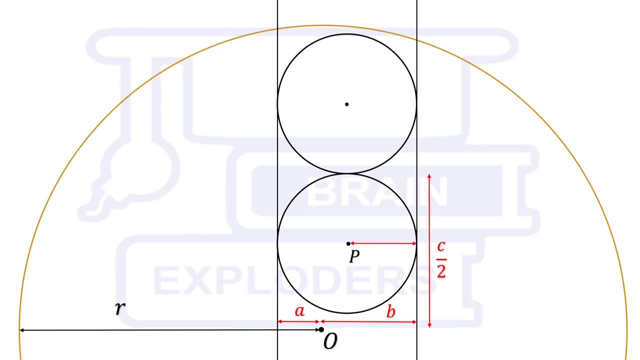 Diameter of these circles is A plus B, so radius is A plus B by 2.. Horizontal distance between O and P can be calculated by subtracting this radius from B, and vertical distance between O and P can be obtained by subtracting this from C, by 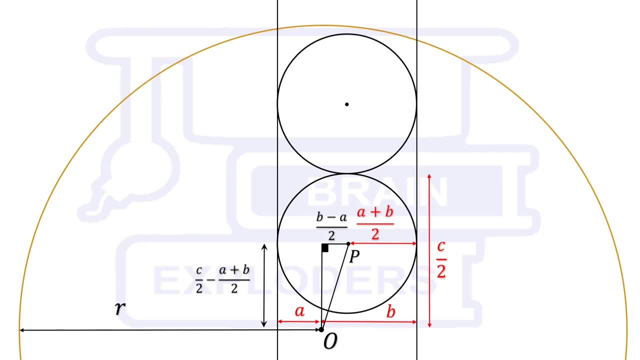 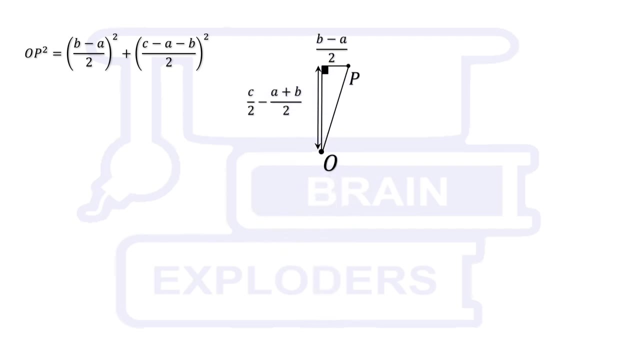 2. These two obtained lengths and OP are together forming right angle triangle. It implies that OP squared is equal to B minus A by 2, whole squared plus C minus A minus B by 2 squared. Center of the circle is at a distance of OP from the center of reference circle and its 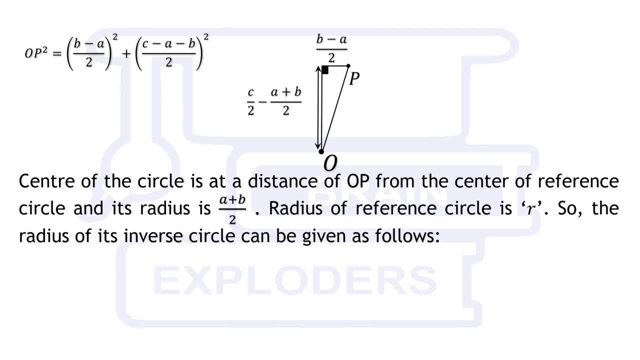 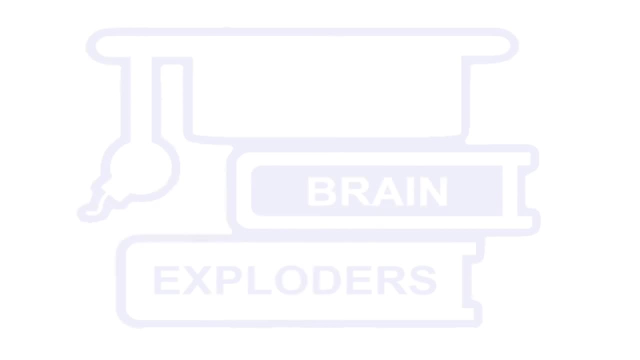 radius is half A plus B. Radius of reference circle is R, so the radius of its inverse circle can be given as follows. That is already discussed in this video On simplifying. we find that 1 over R1 is equal to C minus A minus B, whole squared minus. 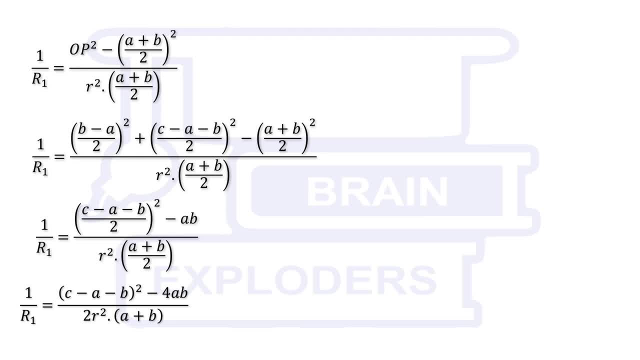 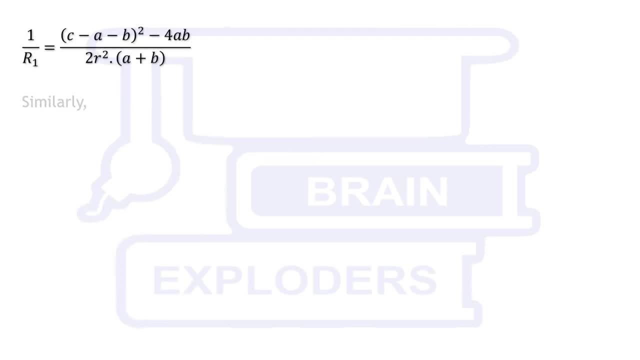 4AB over 2R squared times A plus B. In this way, radius of inverse of other circle can also be obtained by 1 over R2. equals to C plus A plus B, whole squared minus 4AB over 2R squared times C plus A plus B. 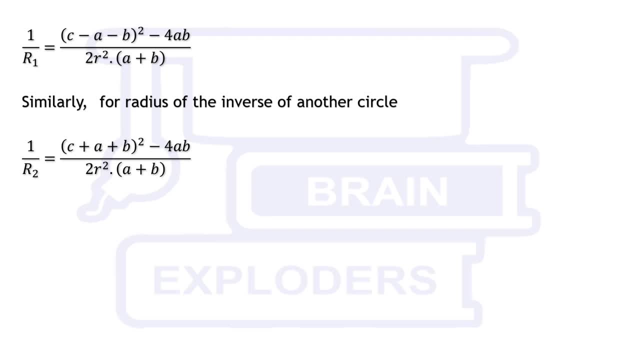 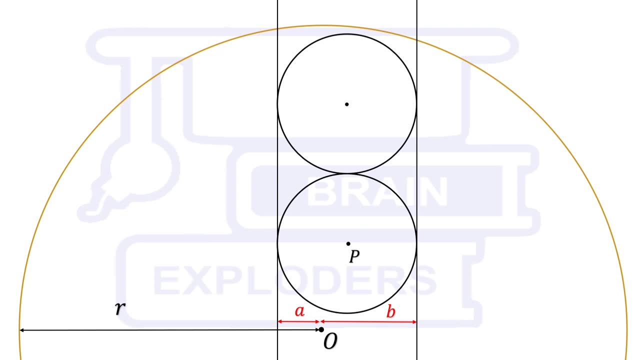 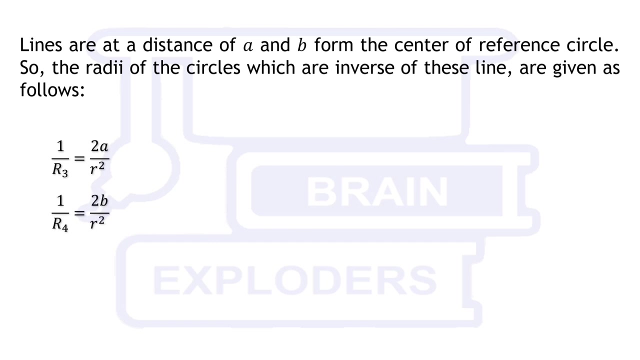 Now we have to find the radii of inverses of these lines. This one is much simple, because distances between lines and center of circle is already available. We get: 1 over R3 equals to 2A over R squared, and 1 over R4 equals to 2B over R squared. 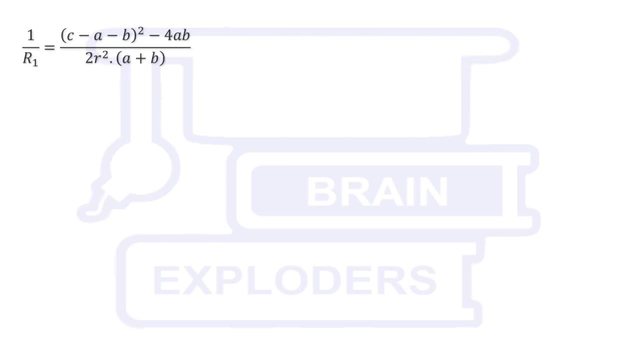 Our goal is to find the relation between R1, R2, R3 and R4. We can say that these are the radii of four mutually tangent circles in parametric form. To find the relation between R1, R2, R3 and R4, we have to eliminate A, B, C and R. 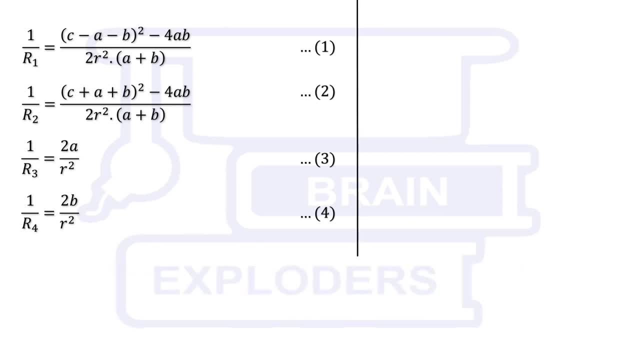 From equation 3 and 4, A and B can easily be calculated in terms of other radii and can be eliminated in any equation. On subtracting equation 1 from 2 and simplifying, we get C equals to R squared over 2 times. 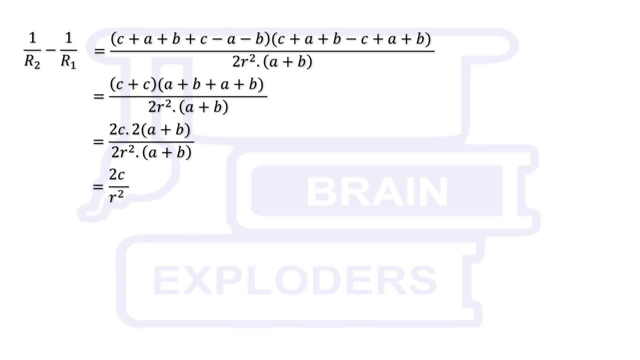 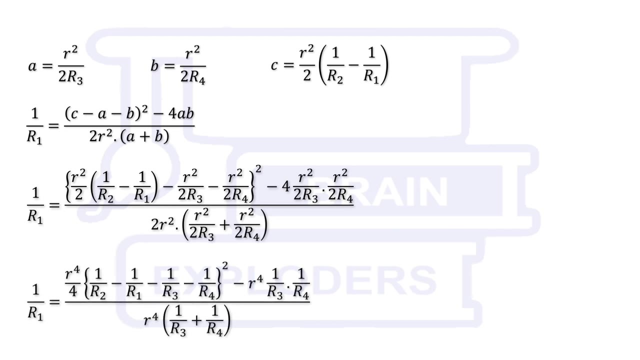 1 upon R2 minus 1 upon R1.. Now put these values of A, B and C in the first equation. R raised to the power 4 is common in both numerator and denominator and it can be cancelled. Do not expand this bracket.